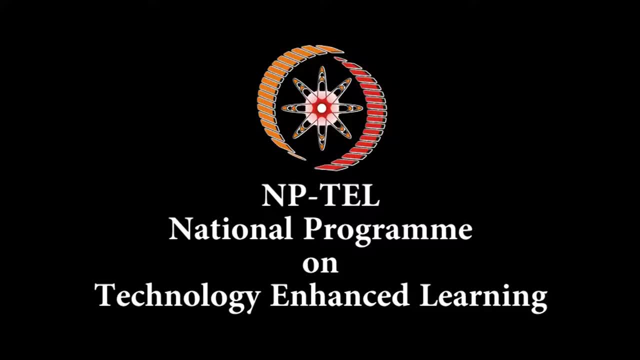 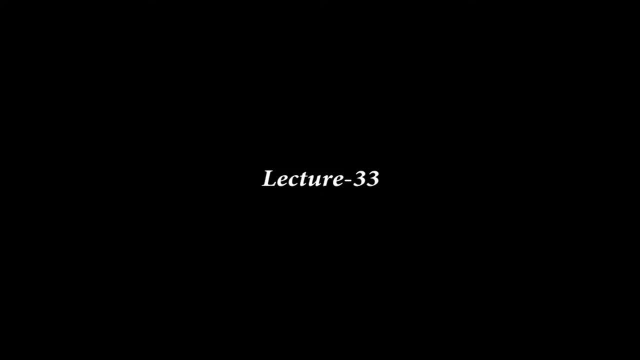 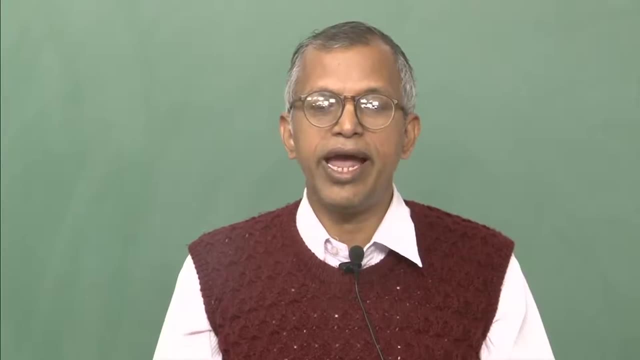 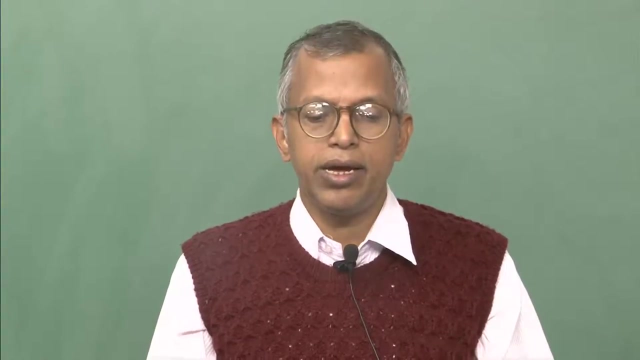 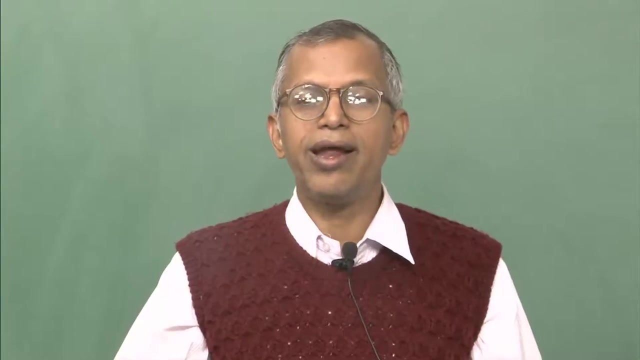 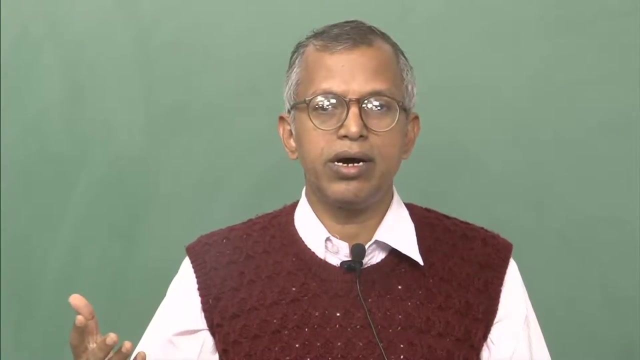 So let us start this lecture 33 and, as usual, we will recall what we learnt in the last lecture. We basically looked at the why we will go for real cycle analysis and how to handle the losses, in case of ideal, in the losses incurred in the engines and incorporate in 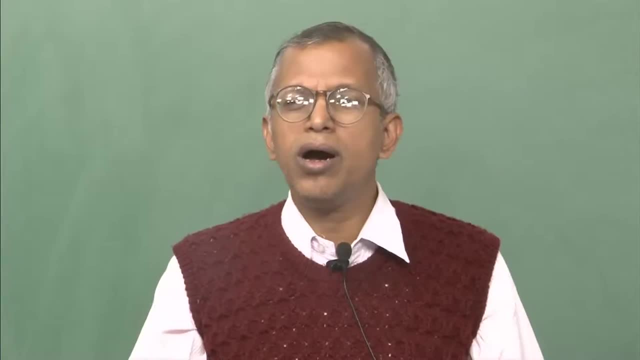 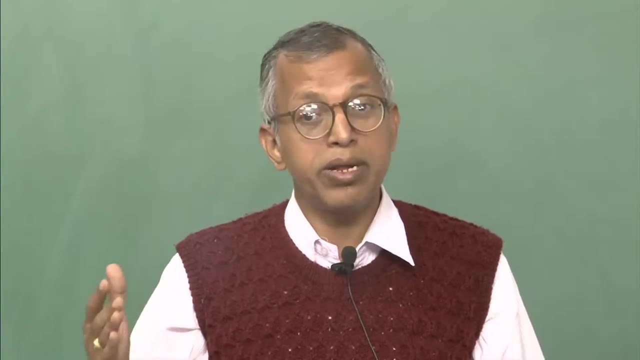 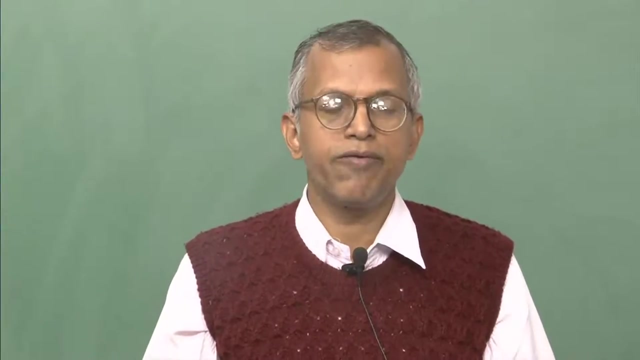 the ideal cycles, such that it will be almost closer to the real cycle in an aircraft engines Integrated engine. I mean only for the gas turbine engine. So what are the those things? we have looked at various components. For example, we have defined the pressure recovery. 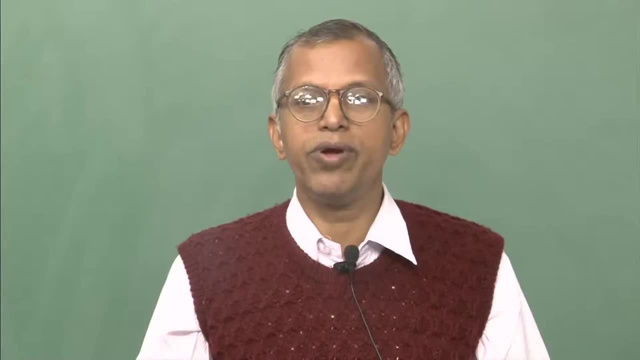 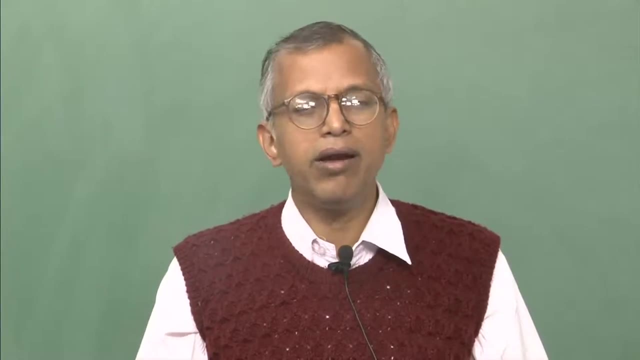 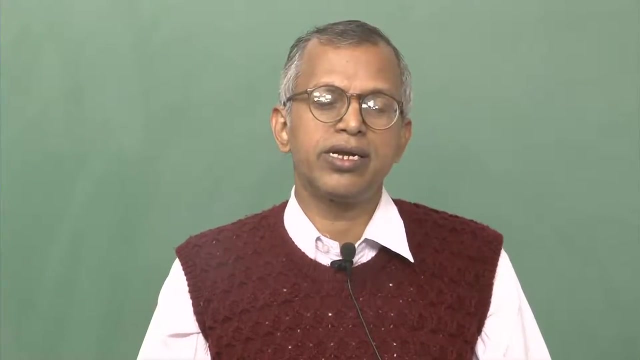 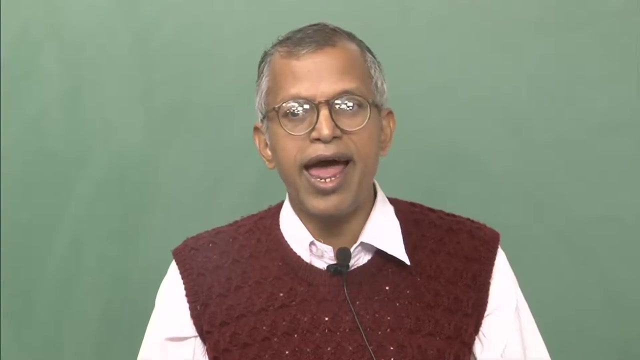 factor in case of an air intake, Then we have also looked at isentropic efficiency for air intake and for compressor turbine. but then we also looked at that it is not good enough to use Isentropic efficiency, particularly for the compressor and turbine, and we will be using 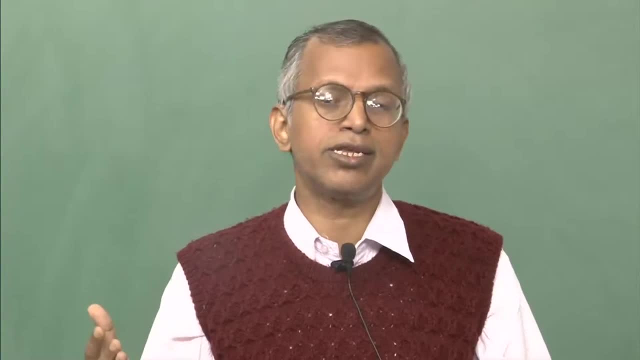 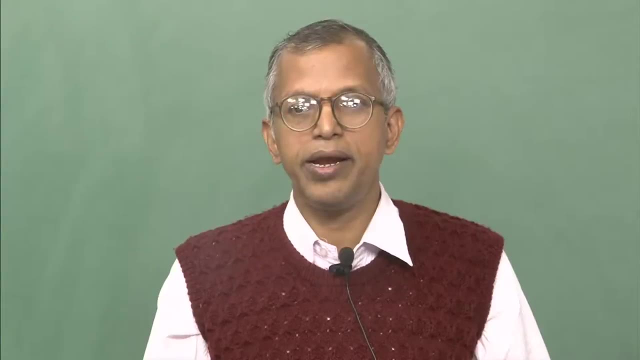 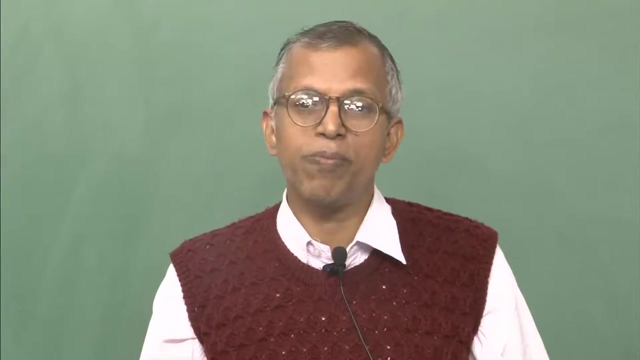 polytrophic efficiency and note that we got a relationship how you can relate the polytrophic efficiency with the isentropic efficiency. But, however, in case of the nozzle and air intake we will be using the isentropic efficiency, but that is not really paying very much. So 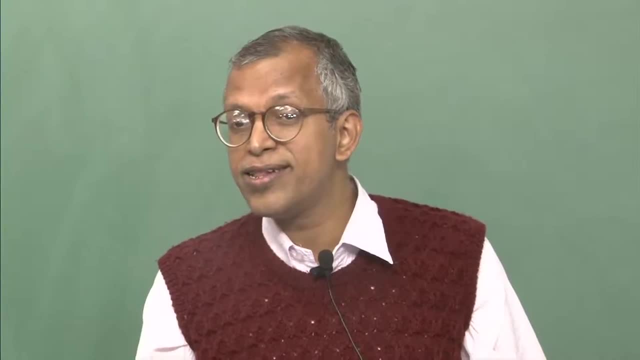 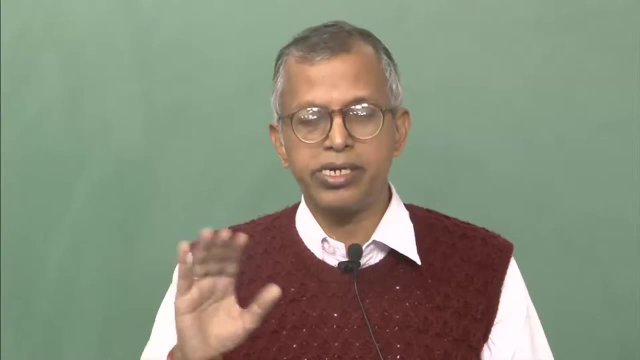 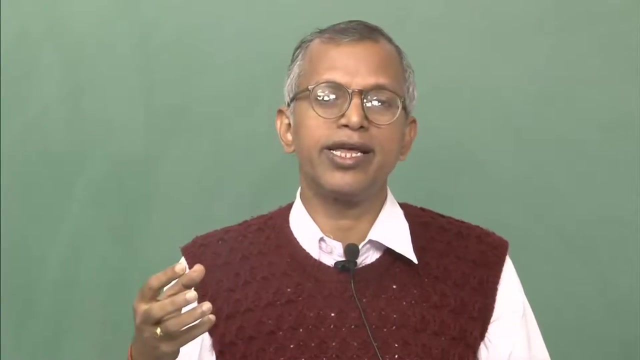 we will be using polytrophic efficiency in very major role. why? because the heat addition or the heat extraction is not there except during expansion and compression. like that is the not extraction, rather it is being changed In case of compression and turbine. you are getting some work done in case of turbine and you are giving work to the fluid or the